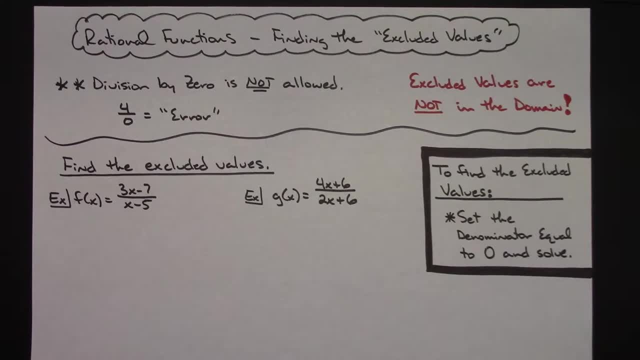 Today I want to take a look at finding your excluded values when you have rational functions. So before we go about doing this, first of all, as soon as you hear rational functions, you should be thinking: oh, it's going to look like a fraction. 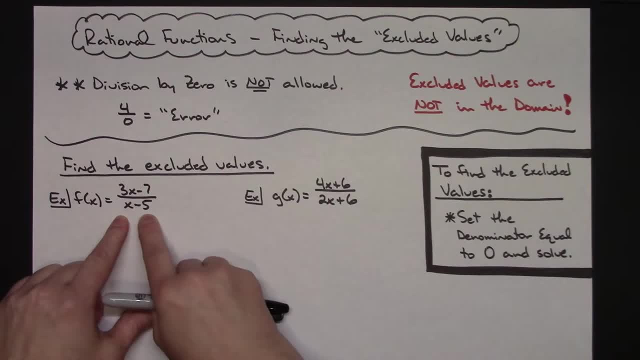 So I've got an example down here: f of x equals 3x minus 7 over x minus 5.. That's a rational function. It looks like a fraction. So particularly we really have to pay attention to our excluded values on this. 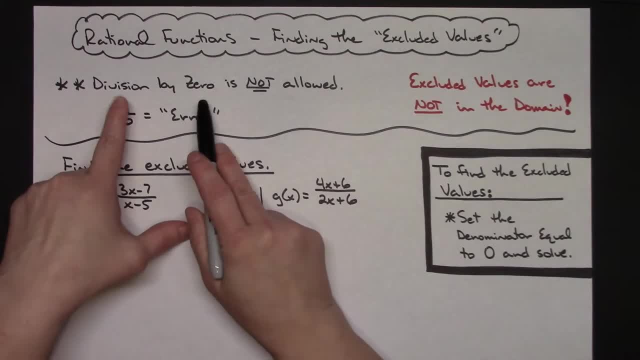 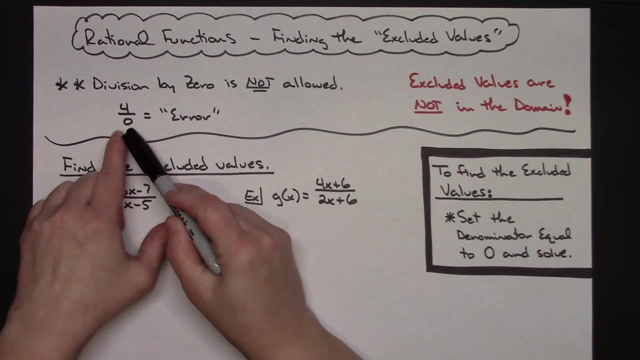 and that's because in a fraction like this we cannot divide by zero. So division by zero is not allowed. You do this on your calculator. If you just take 4 divided by zero, when that bottom is zero, you're going to get an error on the calculator. 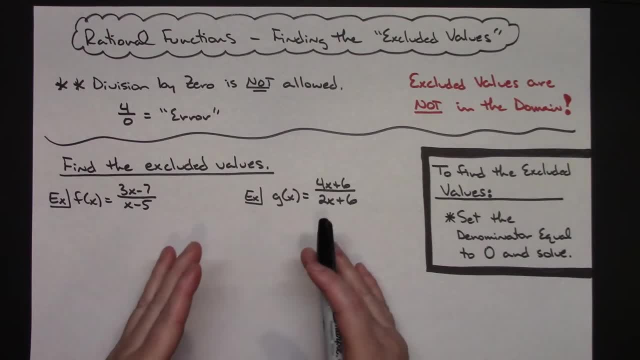 It's just not allowed Now. usually they will walk you through finding excluded values on rational functions, first, maybe in a textbook, and then they'll go on into the discussion of the domain. The reason you're finding your excluded values is because they're not in the 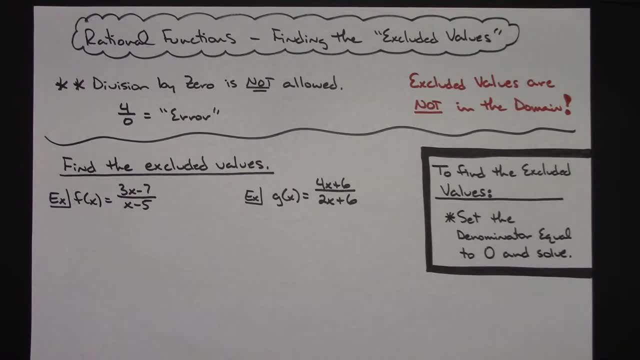 in the domain of the function. all right, And so that's kind of the purpose of just you know, when they just straightforward ask you to find the excluded values, well, they're leading up to you determining the domain of a given function, all right. 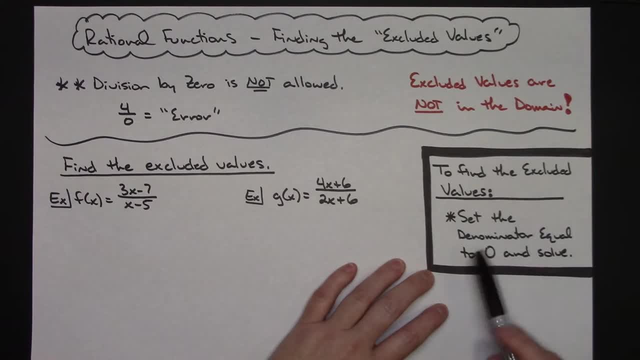 Now over here in the little box, I've kind of summarized your method for finding excluded values when you have a rational function, all right. If you've got a rational function, then all you need to do is set the denominator equal to zero and solve, all right. 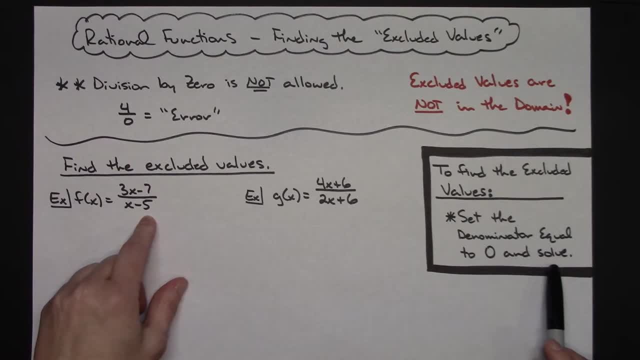 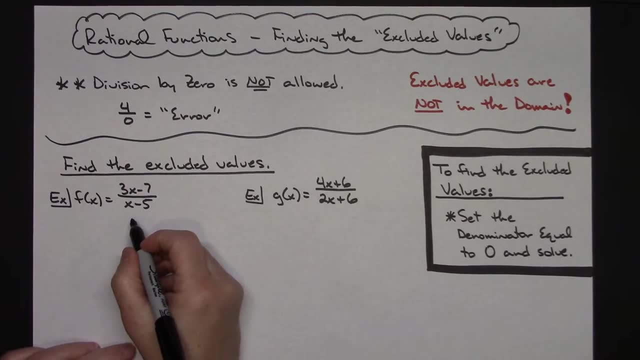 Because then that number, if you plugged it back in, would make that denominator zero, which we cannot have, So that would be our excluded values. So I thought I'd work out a couple examples here. All right, on this first one, I've got: f of x is equal to 3x minus 7 over x minus 5.. 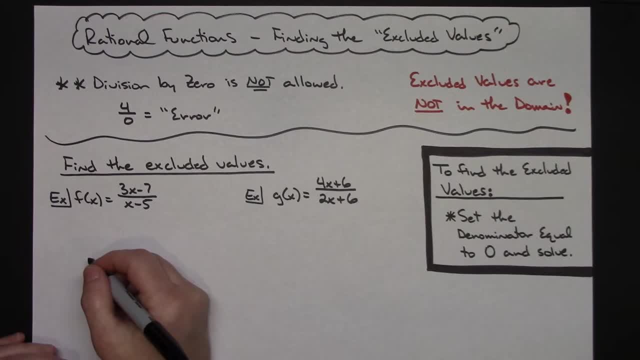 Okay, if I follow my you know process here, I'm going to take that denominator and set it equal to zero. So x minus 5 equals zero. It's a nice little one-step equation. I can add 5 to both sides. 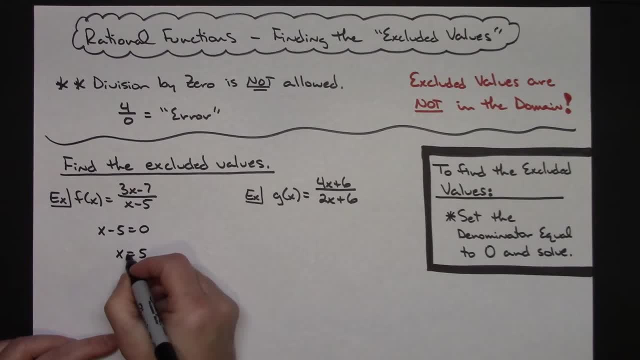 So x is equal to 5, okay when I solve this equation right here, But I'm really going to write this, as x cannot equal 5.. It is an excluded value from my domain. It's an excluded value because if I let x equals 5 and I plug that back in there, I would get zero.